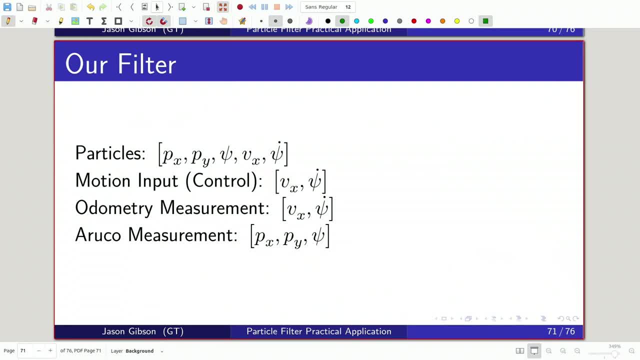 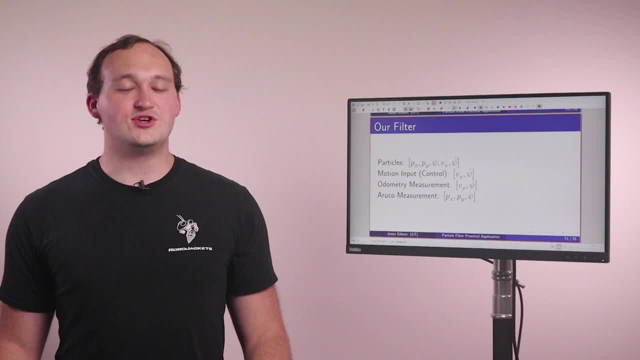 and those will give us a reading on the position of the X, Y and the yaw of the robot. So often you're not going to see things as nice as this particle filter because we have a direct measurement on every part of our state. Often we won't have direct measurements on our states. 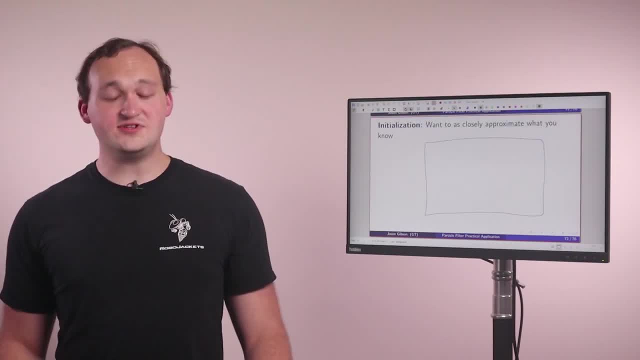 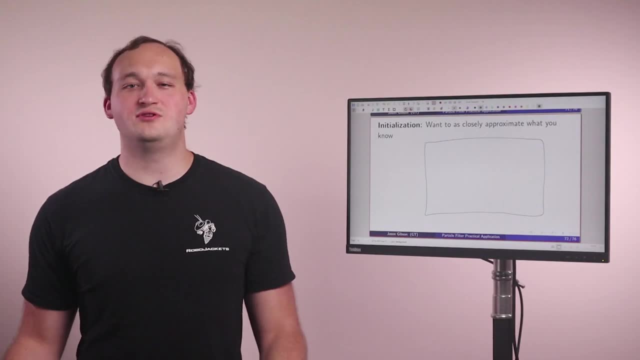 and we'll have to infer them through other parts of the state. So the first issue that you run into with particle filters is okay, cool, I have a bunch of guesses. Well, how do I set up those guesses initially? What should be the initial measurement? What should be the initial measurement? 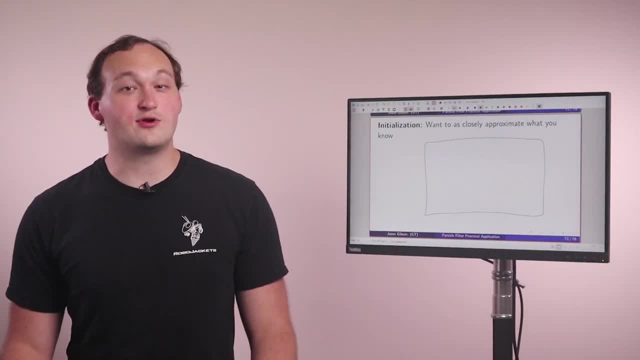 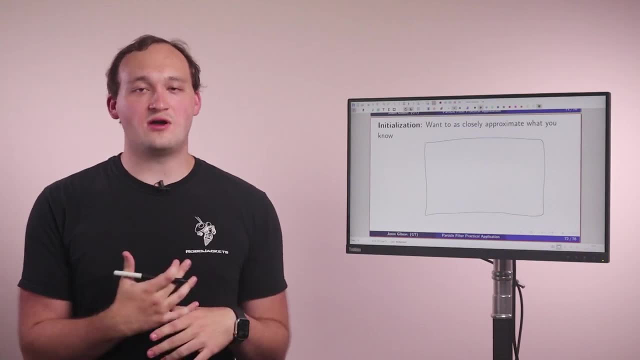 What should be the initial distribution of those guesses. So that depends a lot on your application. So for our application we're in a 2D plane and our robot can have some essentially position and it's going to have some yaw. but we can pretty much assume that our velocity in the X and our 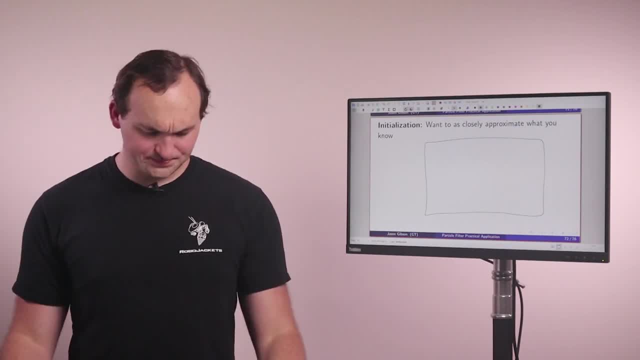 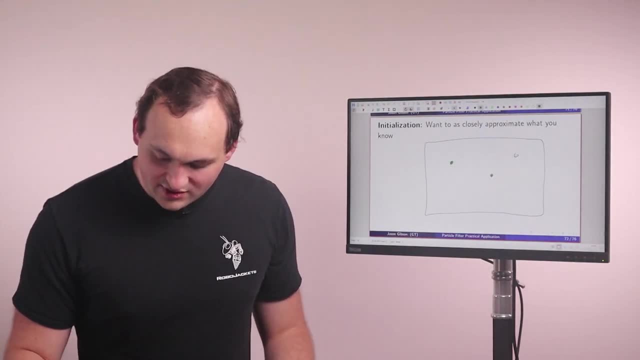 yaw rate is going to be zero because our robot's not going to start moving. So what you want to do is essentially set up particles around the entire course. So you just want to put these particles all around, And the reason we're doing this is because we have nothing that tells us where our 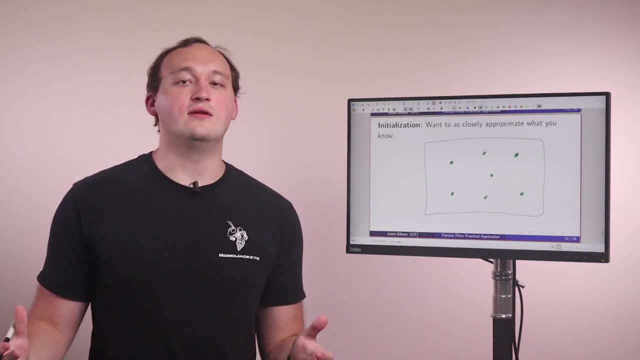 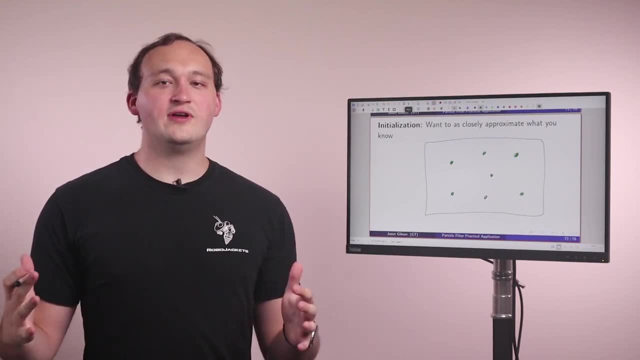 robot should be. All we know is that it should be on this plane. Therefore, it is equally likely to be anywhere on the plane, and that's how we initialize our particle filter. Our particles start all over and then, over time, they'll converge to our actual state estimate. So the next thing we 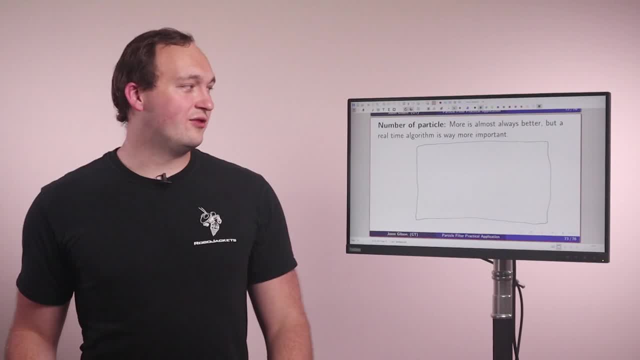 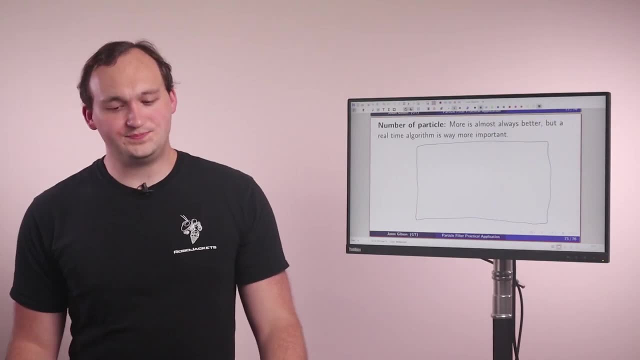 talk about is the number of particles. So the rule with particle filters is more is always better, but honestly, a real-time algorithm is way more important. So it's not really helpful to have a really accurate state estimate if it can only talk you where you were an hour ago and can't tell you where you are right now, because oftentimes you 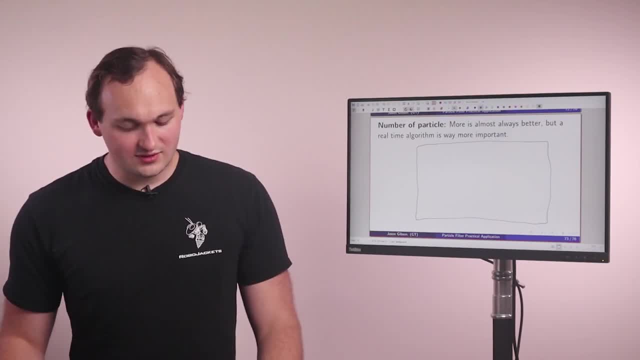 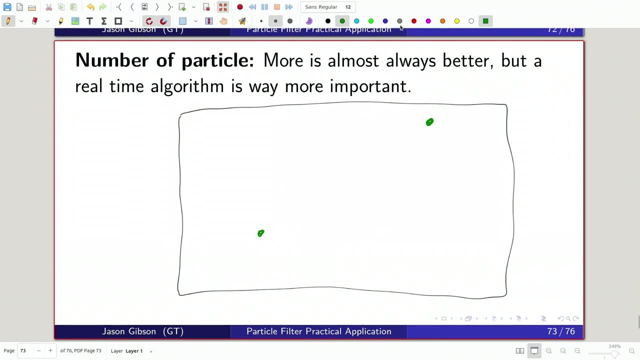 want to make decisions about now and not an hour ago. So the way you can think about this is: if we have too few particles- let's say I have something like two particles and my sensor reading says that I am here- well, both those particles are pretty low probability and there's not really. 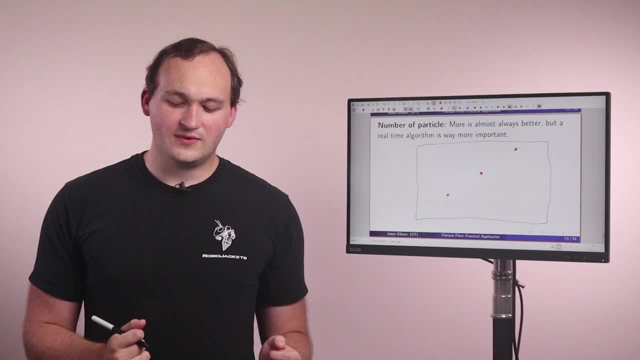 a good chance that they're going to move in the right direction. So we want to have more particles, and essentially what you need is enough particles to cover your state space, but not too many that you slow too far down. There are different tricks to get around this. 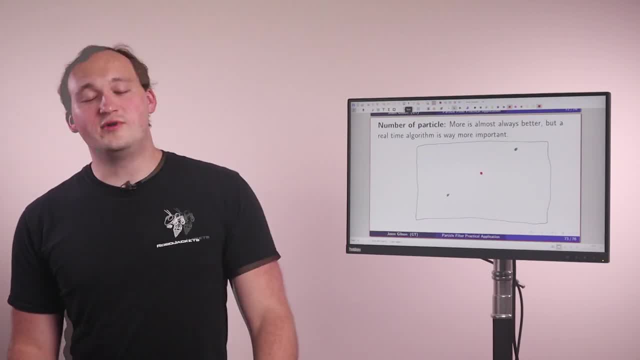 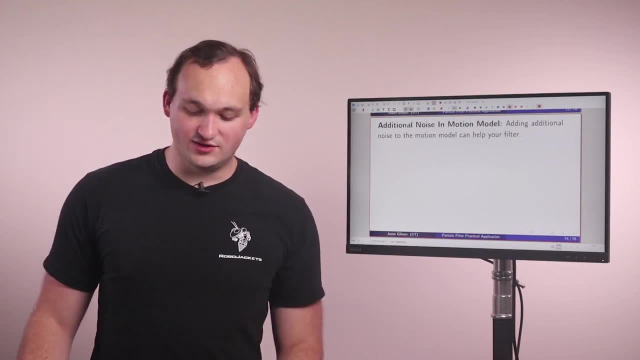 like parallel computation and other things, You'll want to treat number of particles like a hyperparameter and just play around and see what works best. So another trick that you want to add in particle filters is this thing called adding additional noise, and the reason that 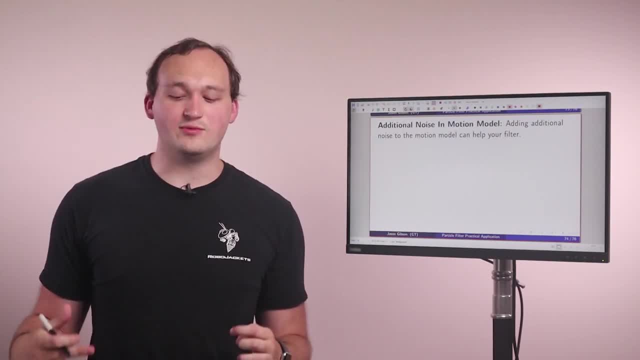 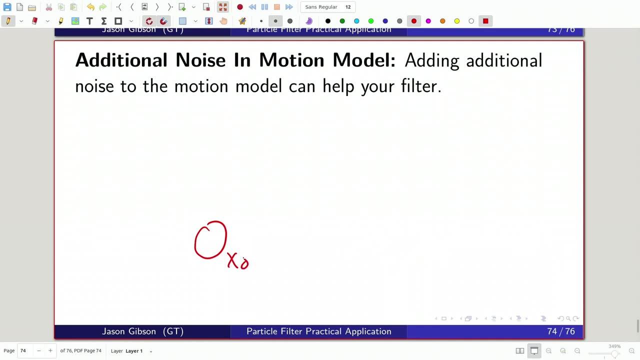 you're going to do this is because it helps the particle filter initially converge and remain with a state estimate, because remember that we don't have perfect estimation of how our robot's moving. So let's say we have some x0, which is our initial distribution. 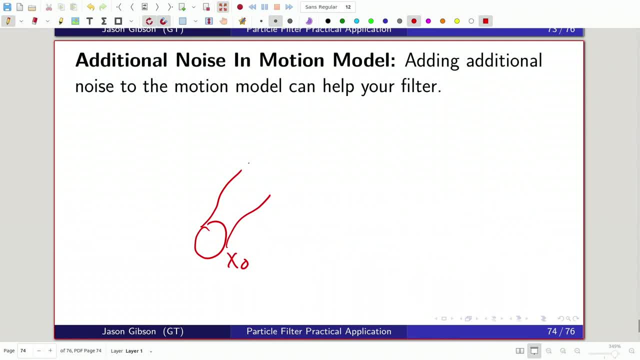 and then what we want to do is: we want to move it. So we're going to move it based on our motion model and we get some larger ring of uncertainty because we have moved, But our sensor model is telling us that we're right here. So what'll happen is, over time, we'll eventually converge to. 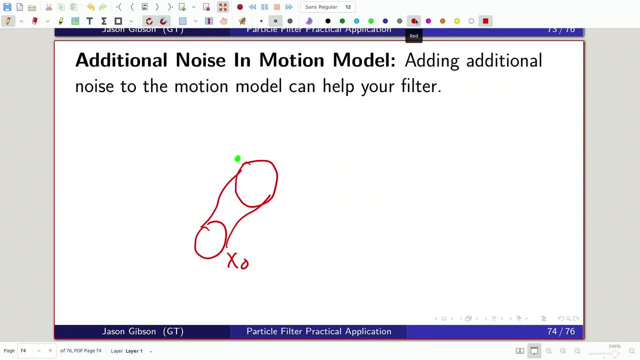 it. Sometimes it's really nice to add more noise than you think should exist in the motion model, because then you'll get some kind of uncertainty like this and it'll tamp down based on your actual sensor reading. So now you'll get some representation like that, which is much closer. 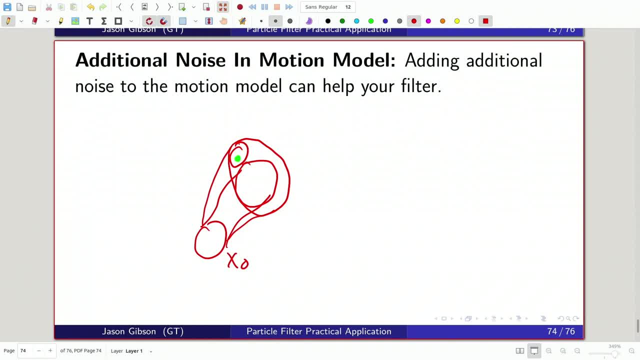 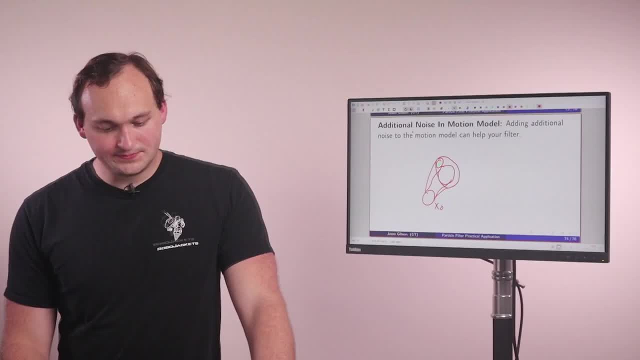 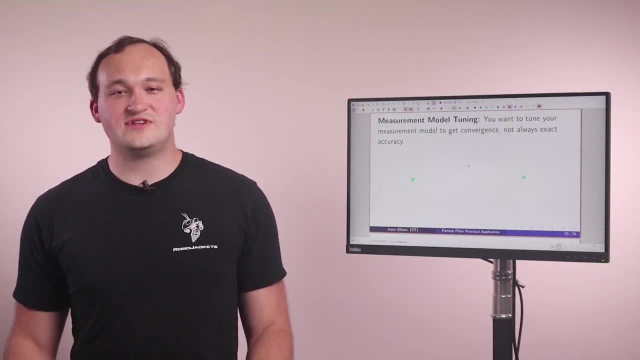 Obviously this is a tuning thing and just to depend on your application And often you can just kind of set it to the right value and see what converges and play around with it. So the other thing to play around with tuning-wise is the measurement model tuning. So, again, just like with the motion model, technical, physical, 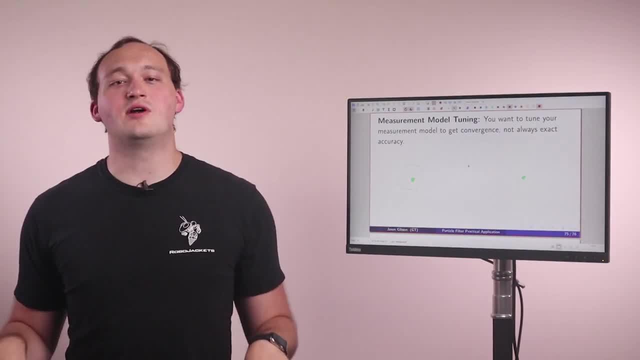 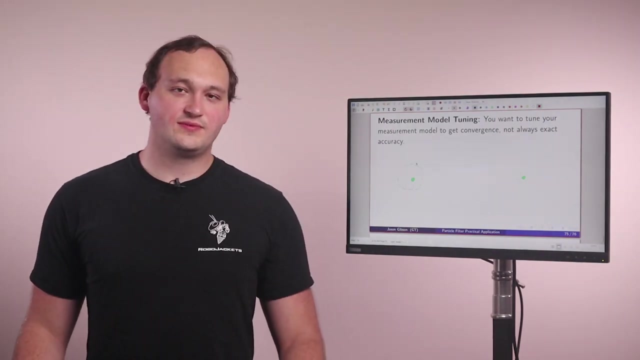 accuracy is not always the goal here, While you want to represent the probability distribution correctly. oftentimes it's better to have a converged filter than a diverging filter, because when your filter diverges you just get nothing useful. Let's talk about a little bit why that makes sense here, Oftentimes with your measurement model. 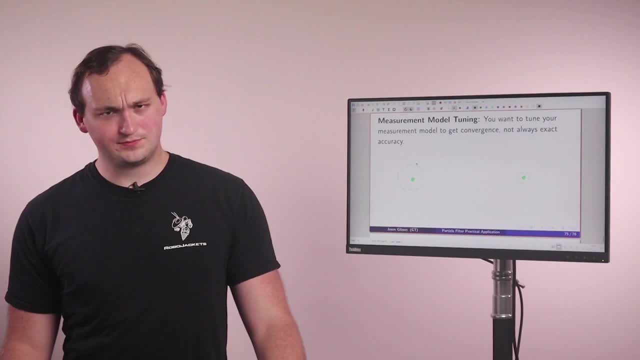 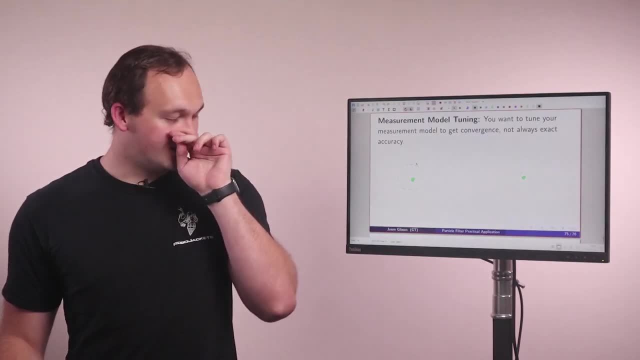 it's helpful to have higher covariance than you think you actually need, because it'll allow your filter to converge faster and be a little bit more stable. So let's say I have the two representations here. So over here I have what is actually true. 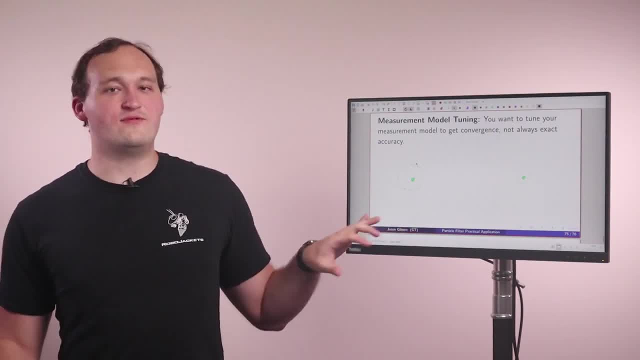 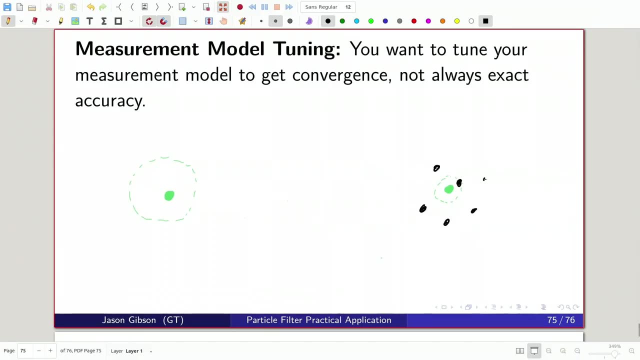 what is my sensor reading telling me how accurate it is? and here I have one that's a little bit larger, And what's helpful about this is, if I have particles like this often you get a little bit of a difference between what you think is correct and what's not. So if you're 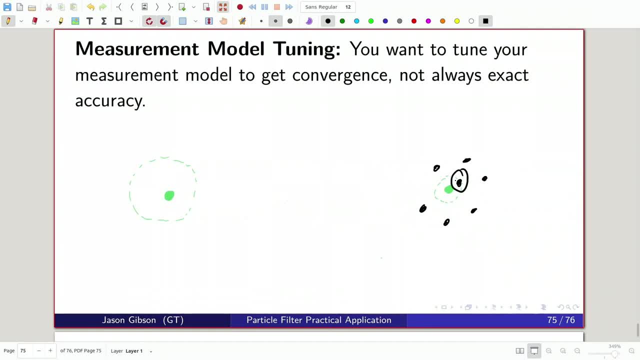 going to get into numerical issues, because only this one is really probable, given our sensor reading. the other ones are still pretty close and this will often result in some numerical instabilities. We can increase the covariance and by doing so we'll get a little bit smoother convergence of 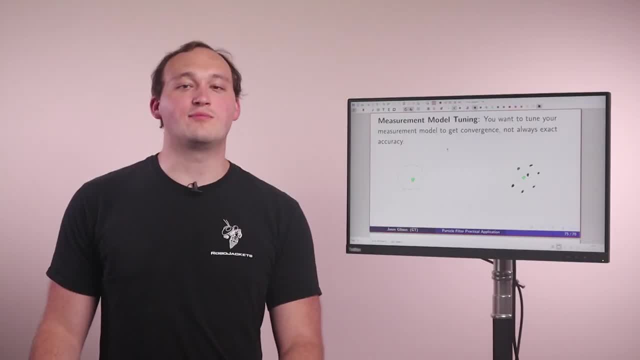 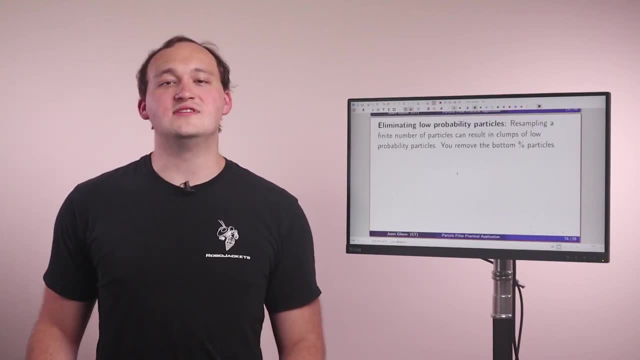 our particle filter. Playing around with the measurement covariance is often a good way to make a particle filter work better. The final trick, which is kind of a hack and really just due to problems in numerical stability: reducing low probability particles. So essentially, what I'm going to do is I'm going to